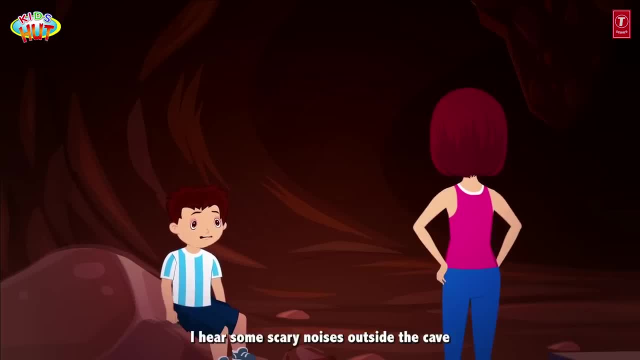 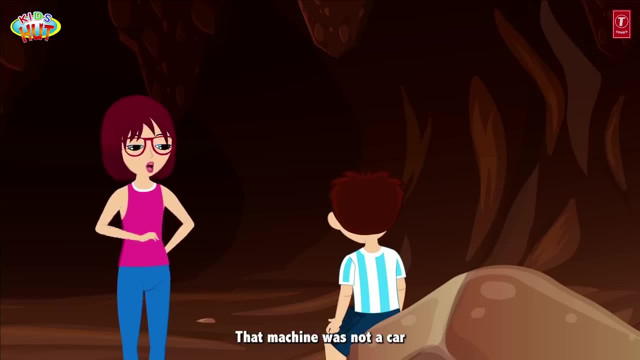 Tia, where are we? I want to go home. I hear some scary noises outside the cave. I hear some scary noises outside the cave. Tofu, that machine was not a car, It was a time machine. It was a time machine. 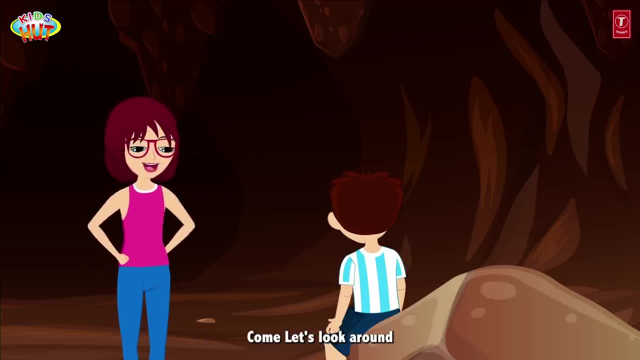 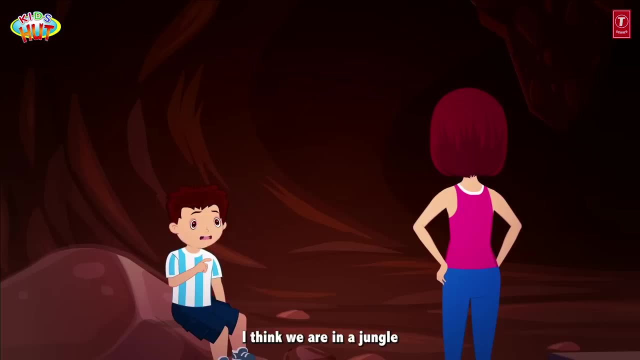 It looks like we travelled back in time. It looks like we travelled back in time. Come, let's look around. I feel so scared, Tia. I feel so scared, Tia. I think we are in a jungle. There are wild animals outside. 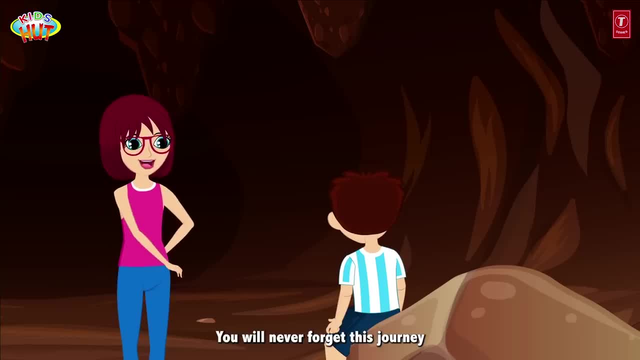 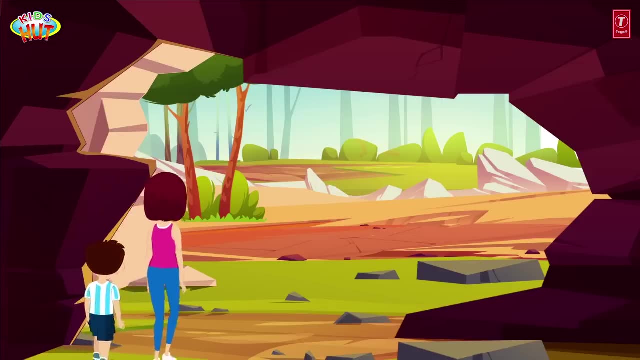 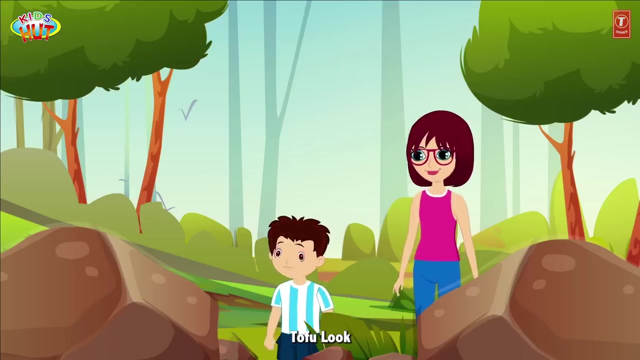 Tofu, trust me and hold my hand. You will never forget this journey. You will never forget this journey. Okay, let's go if you say so. Okay, let's go if you say so, Tofu, look. 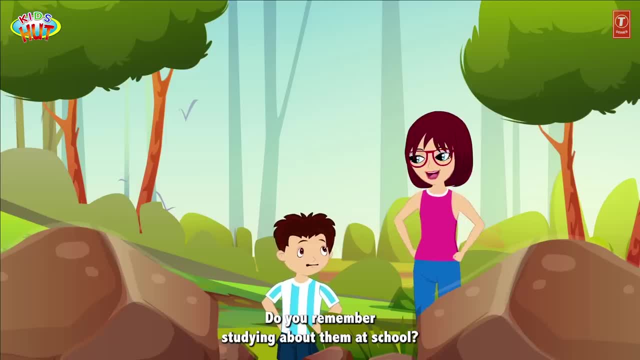 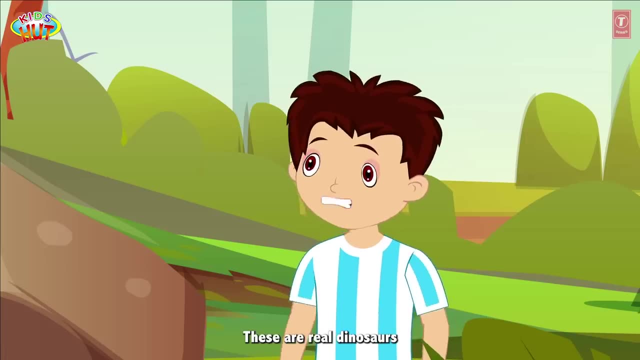 Tofu. look, There are dinosaurs. Do you remember studying about them at school? Do you remember studying about them at school? I can't believe it. These are real dinosaurs. They look so scary. Tia, What if they come and get us? 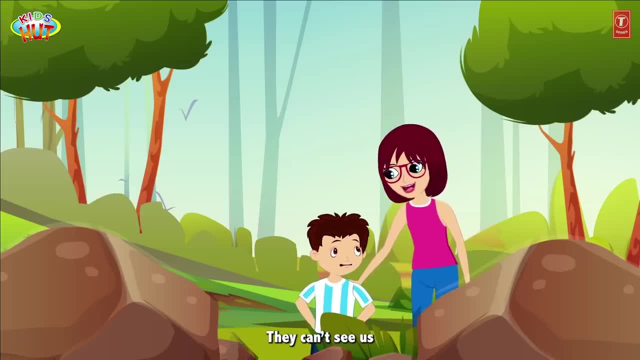 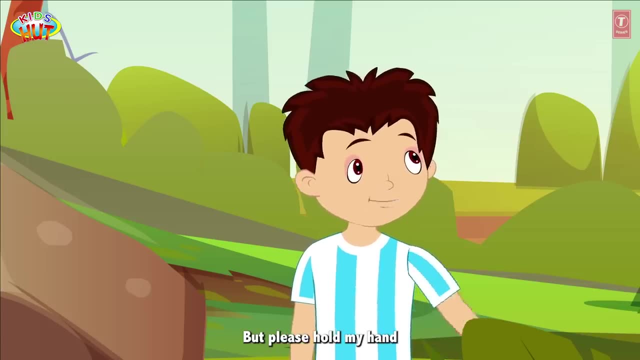 What if they come and get us? Oh, don't worry, They can't see us. Do you want to go closer? Okay, let's go. Please hold my hand all the time. Please hold my hand all the time. I can't believe my eyes. 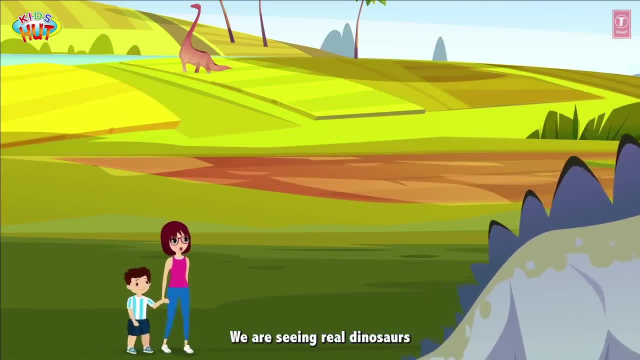 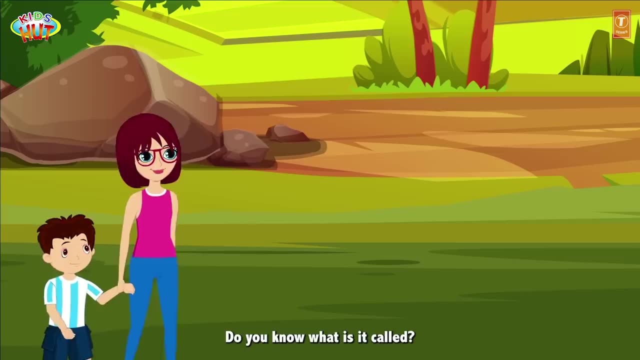 I can't believe my eyes. We are seeing real dinosaurs. We are seeing real dinosaurs. Look Tia, that dinosaur is so gigantic. Look Tia, that dinosaur is so gigantic. Do you know what is it called? Do you know what is it called? 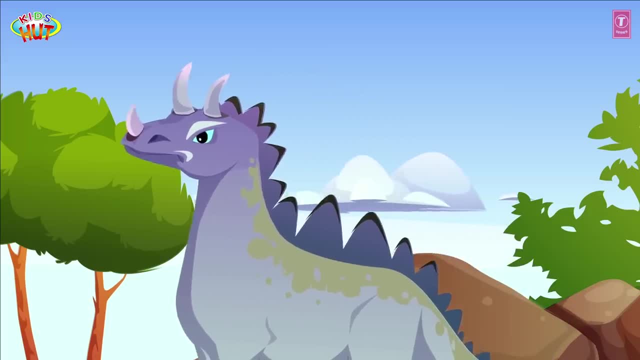 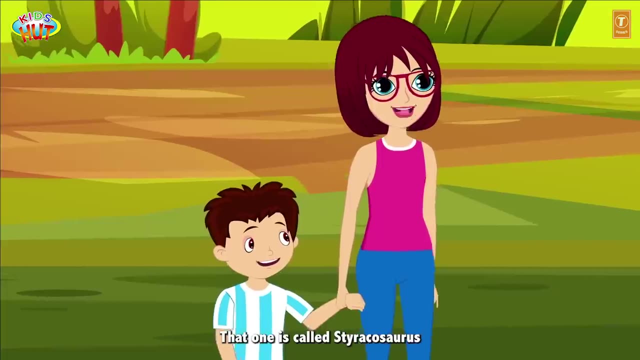 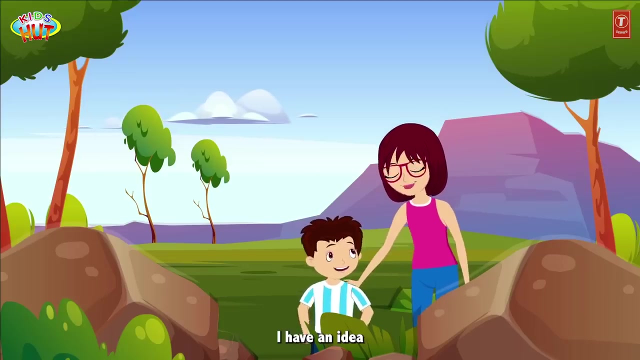 That's a Carnotaurus. That's a Carnotaurus. Oh, I see a dinosaur with horns. That one is called Arachosaurus. They have such long and funny names. They have such long and funny names- Tofu. I have an idea. 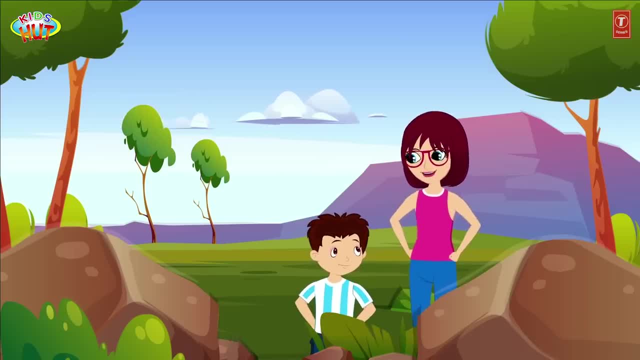 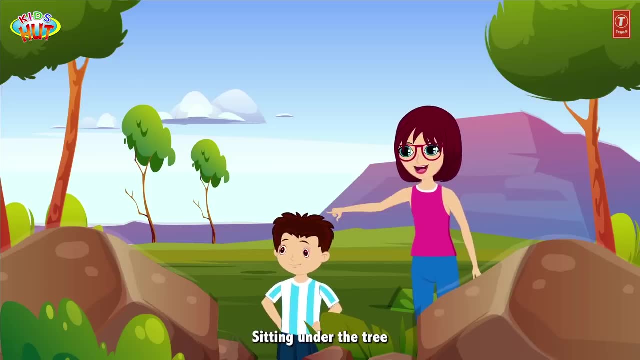 Do you want to ride a dinosaur? Do you want to ride a dinosaur? Ride a dinosaur. How is that possible, Tia? Look at that one sitting under the tree. Look at that one sitting under the tree. Come, let's climb its tail.